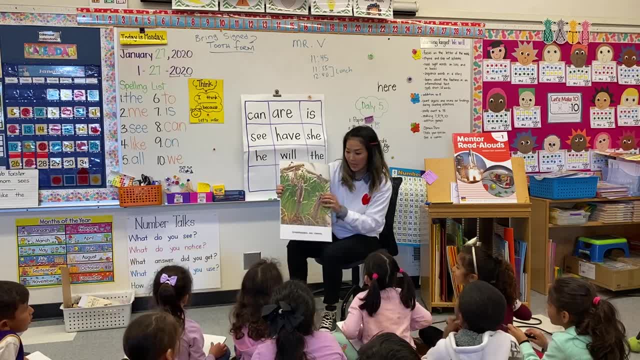 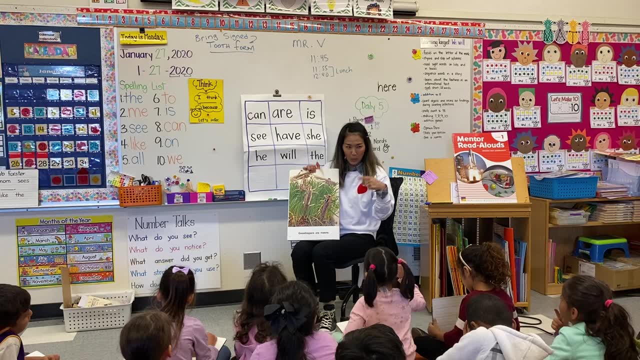 Right, Okay, okay, So we'll make it match first here. Okay, So here we'll say they are brown and black. What do you guys think? Yes, Okay. Well, let's count, like in the morning when you guys are doing some sound together with Ms Forster. 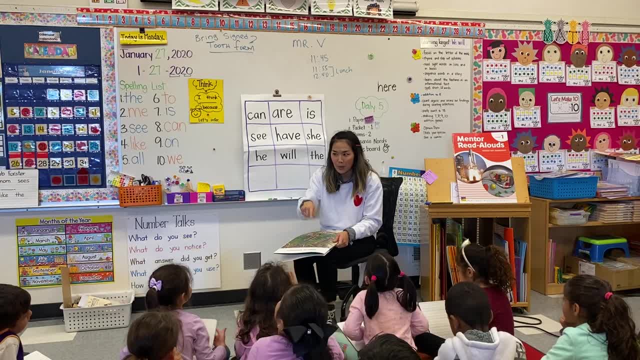 Let's count how many words. How many words are in that sentence? Ready? So show me your hand. like this, We're going to say they are black and brown. Are you ready? Let's count how many words Go. 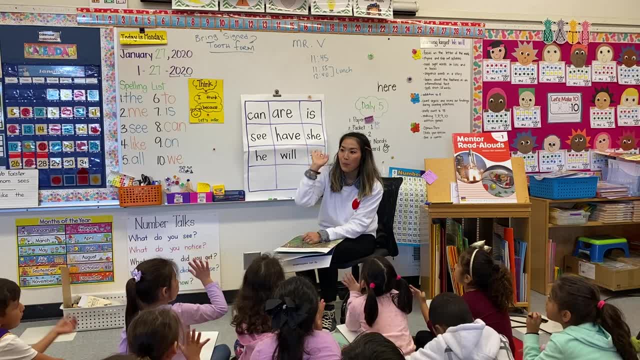 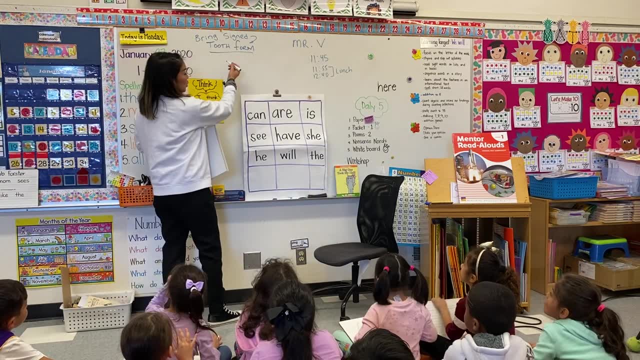 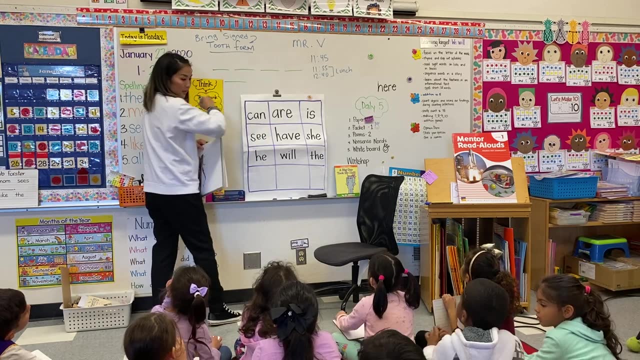 They are black and brown. How many words is that? Five, Five. So on your board, can you do this? Can you draw five lines: One, two, three, four, And if you have to go to the next row, you can. Can you just do that for me? 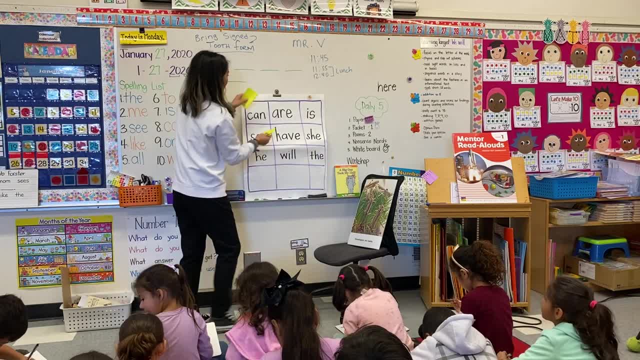 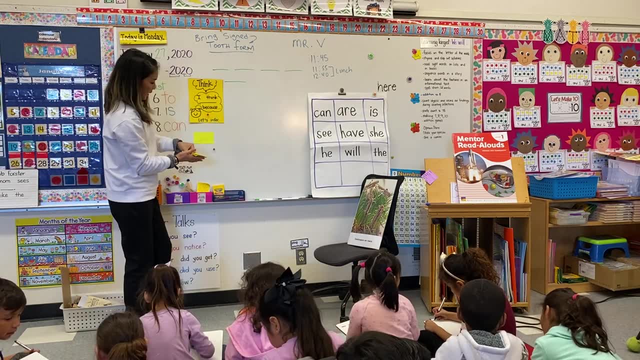 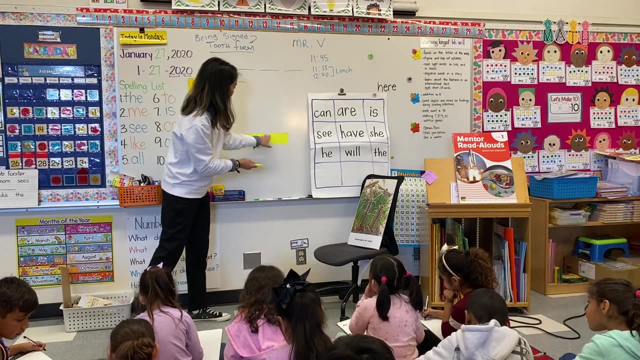 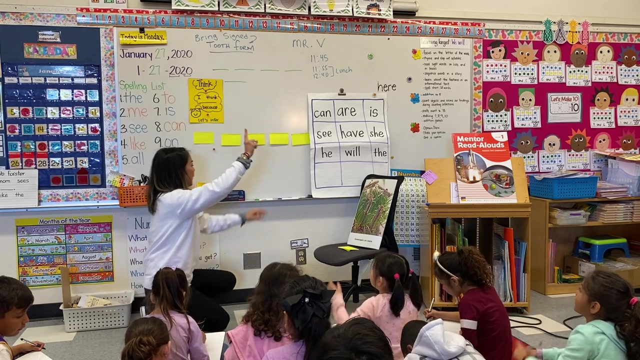 One, two, three, four. Now you ready, Ready, Okay, Here we go. One, two, three, four. One, two, three, four and five. Okay, So you ready. Can you show me your pointer finger or your marker? 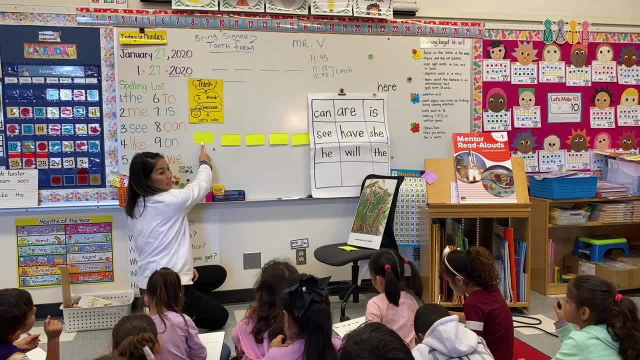 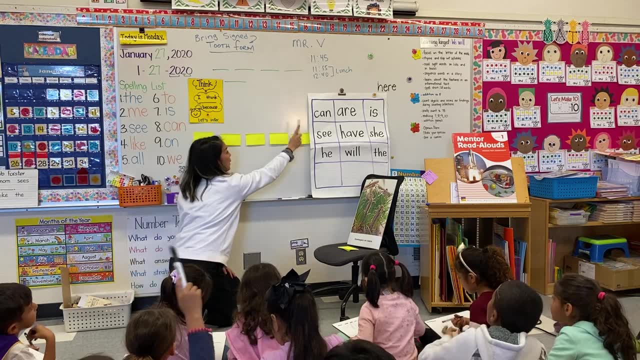 You can do this with Ms Courtney. You ready? Yes, Tell me what words you're going to write down. Yes, I'm going to write it here. You ready, Go Five. They are black and brown. Can you repeat it again? Ready, Go. 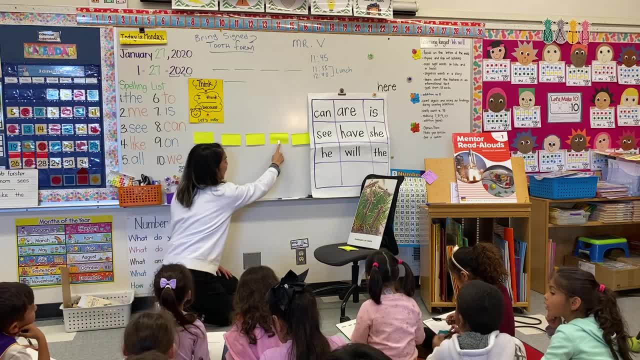 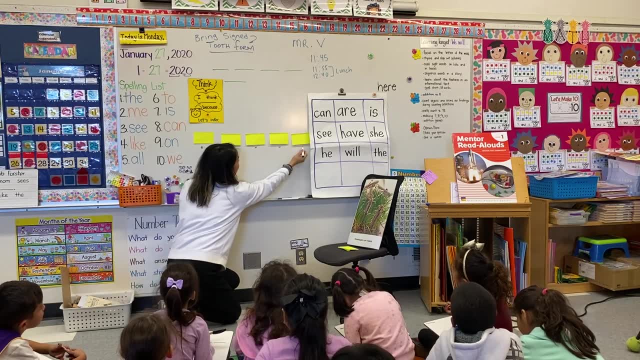 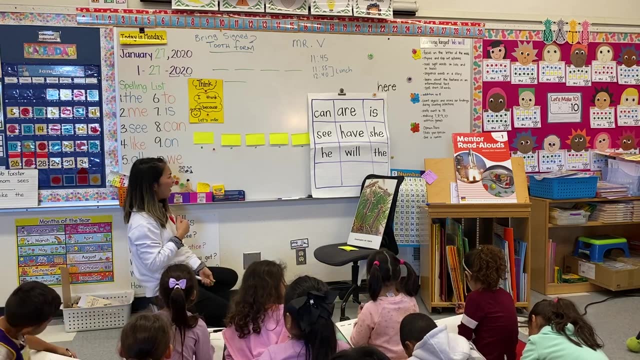 They are black and brown, Awesome. So Ms Courtney is just going to put these little dots underneath that we know to match our fingers right, Our words to what we're saying, to match it. So they Huh, They, Hmm. 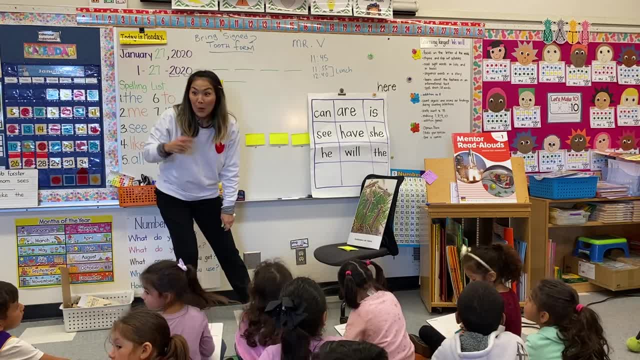 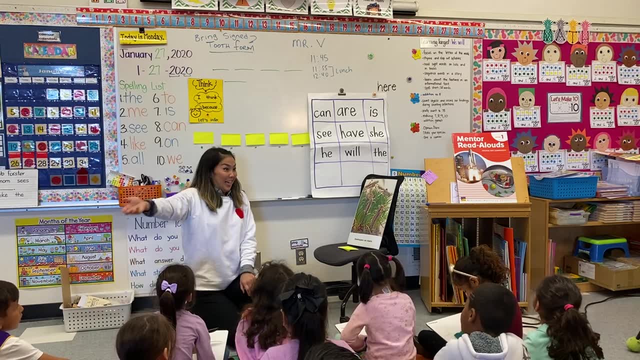 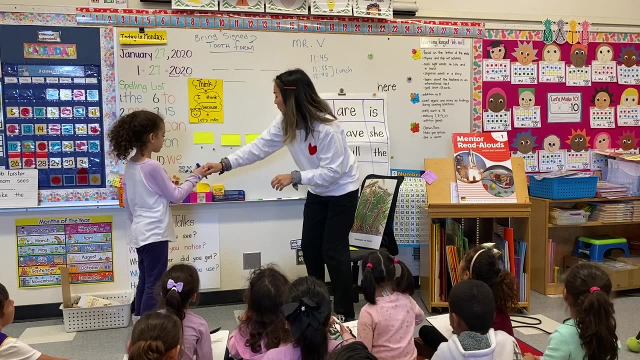 Where's my friend Logan? Logan, Logan, Do you hear that th? th in they? What two letters make a th th, th, T-h, T-h. Logan, come on down, T-h Boys and girls. do I see a T-h? Here we go. Logan, can you do a T-h for me? 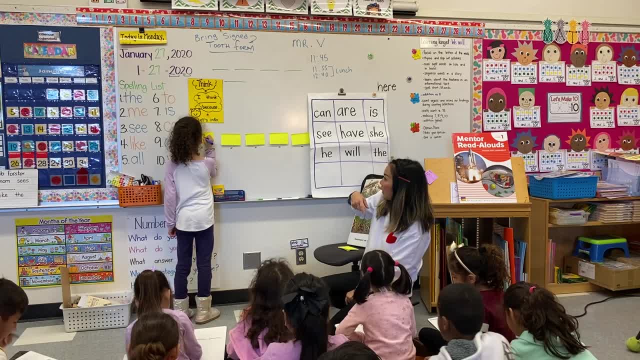 Boys and girls. can you write T and an H on your board too, like Logan? You just T-h, Logan. I got the rest. Thank you, You got it Okay, Thank you, Thank you. Thank you, It's okay, Thank you. 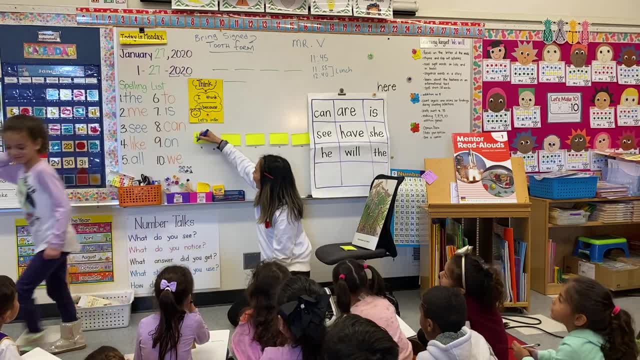 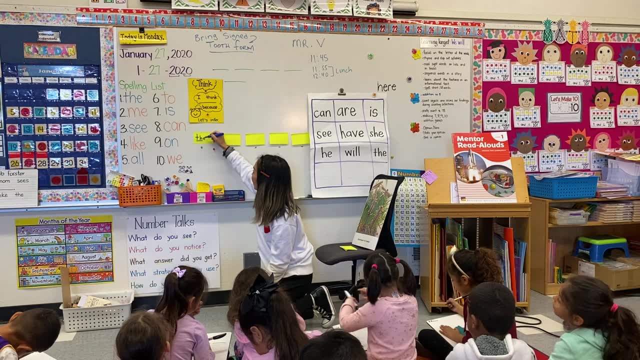 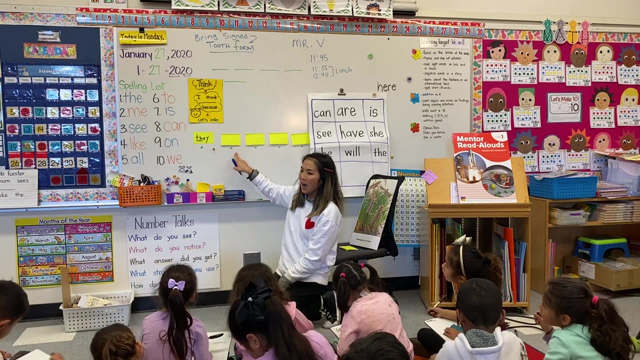 Good job, It's okay, Thank you. So here, right, Did everyone do T-H? I hear it T-H? right, Ms Quentin's going to take care of the rest. They, they are. I think R is one of my high frequency words. 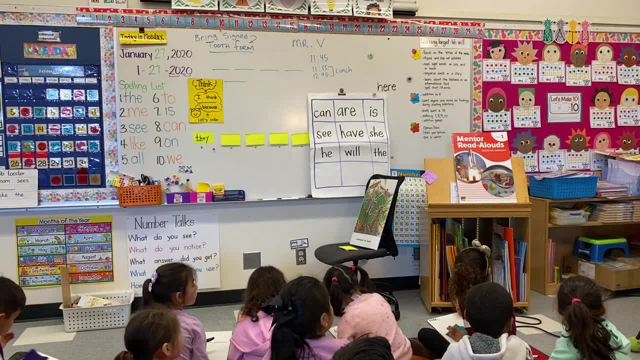 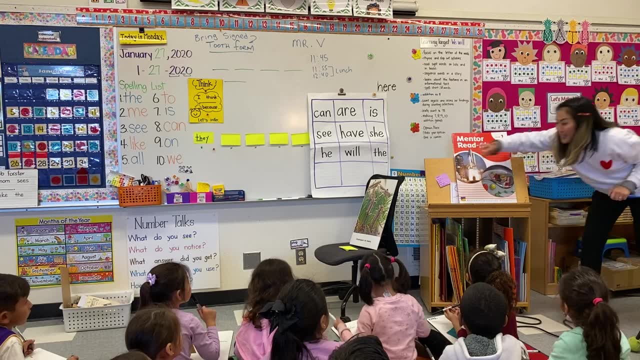 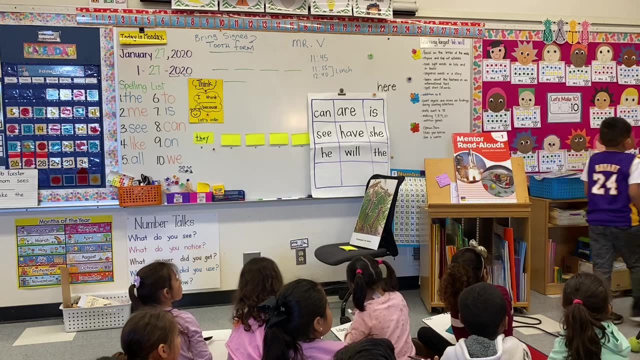 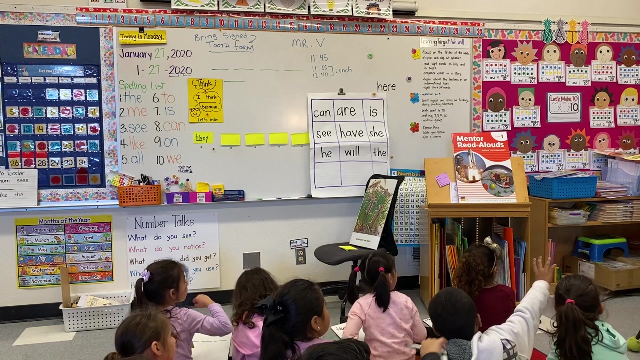 Oh, my kindergarten friends, Look, Do you see it somewhere here? Yes, Oh, my friend, Vincent. Come on down, Where's Vincent, Come, come, come, Hurry, hurry, hurry, Come and show me which word is R, Which one, which one. If you see it, pretend to grab it. Which one is it? Which one is it? Oh, grab it. Got it? Okay, let's go back. go back, You guys got it? Yeah, Okay, ready. 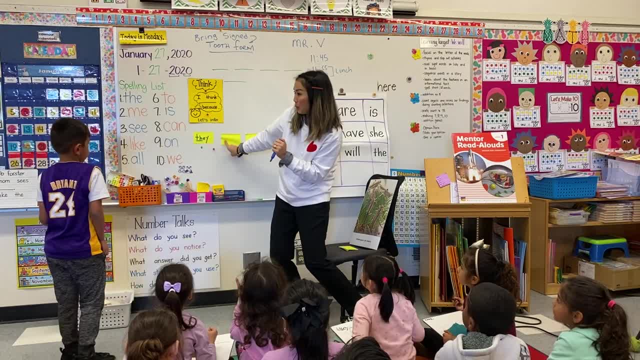 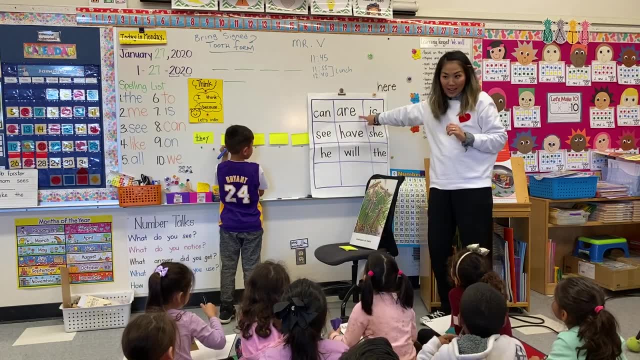 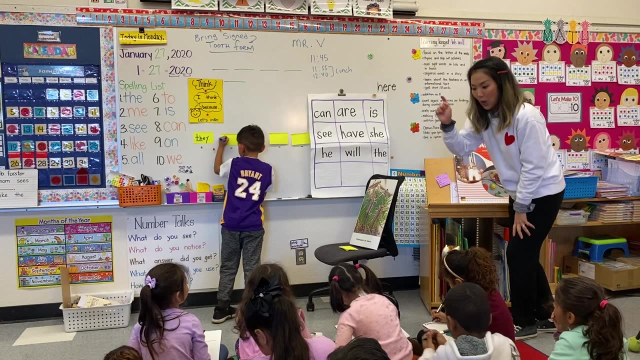 Vincent, ready, You're going to throw it right here, to the next word: Ready, Vincent, Throw it. Okay, here, ready. And if you don't know, look, Ms Quentin found it. here too, You ready. Everyone say A-R-E. Can you say that? A-R-E Say R. Okay, write it Nice. 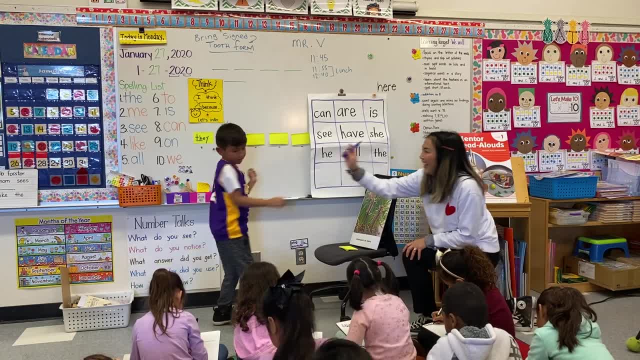 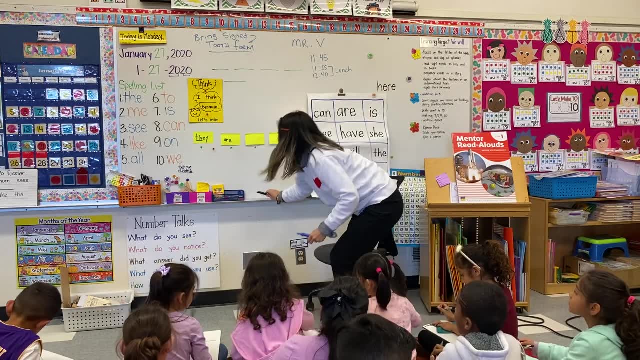 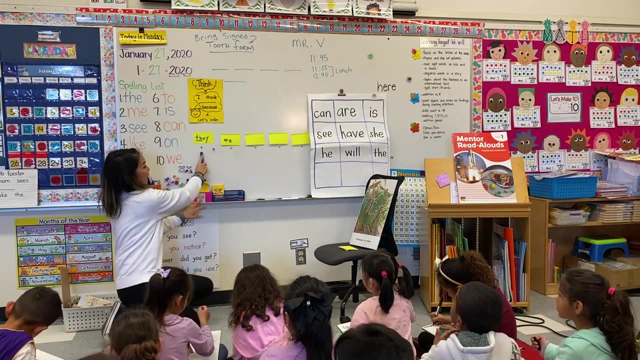 A-R. This mic is not working. Your mic is not working. It's okay, You can borrow this one real quick. Okay, All right, Here we go. Show me your marker Up. Ready, That's point Ready go, Say they. 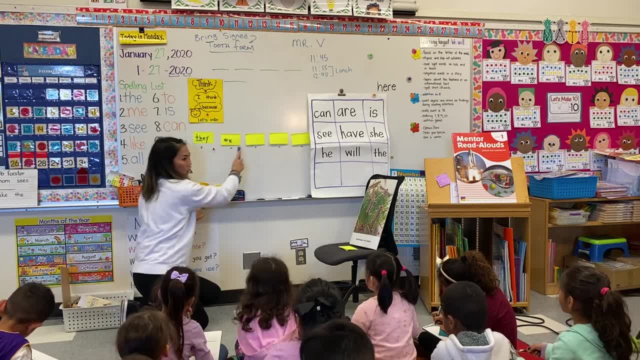 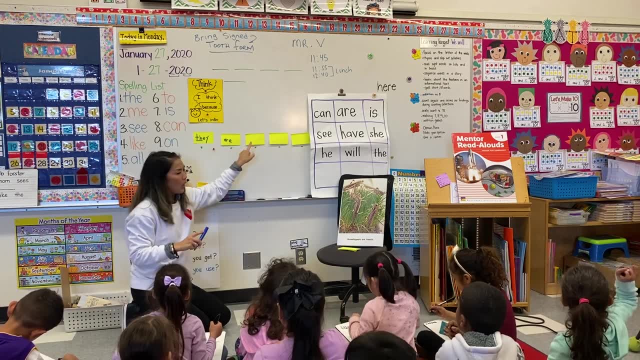 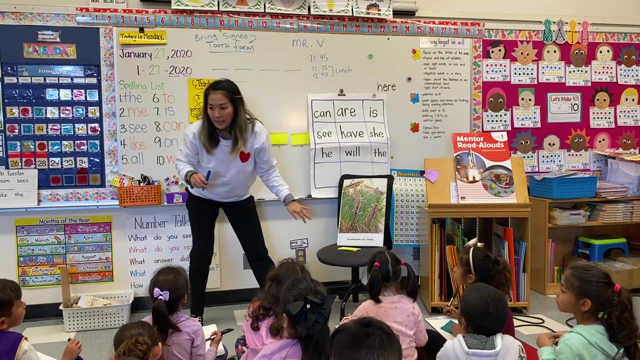 They are. Huh, What color do we say? Brown, Brown, Right, They are brown and black. Okay, Bruh, bruh, bruh. What two letters make a? bruh, bruh, bruh, Cecile, Cecile. Oh there, What two. 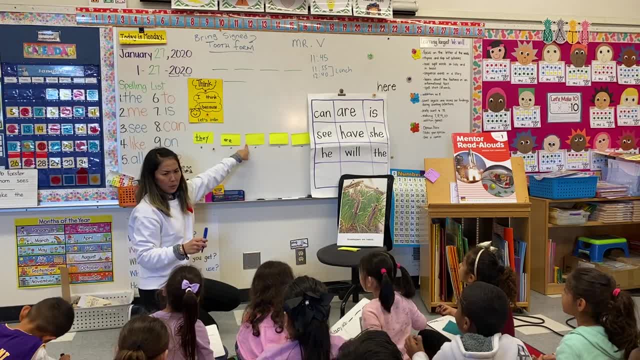 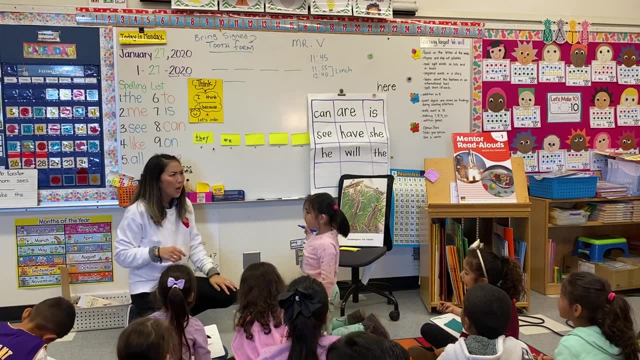 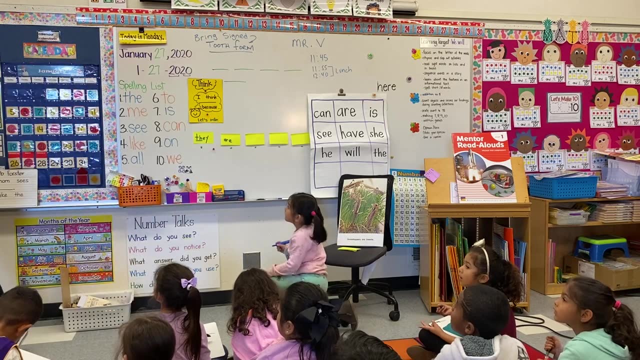 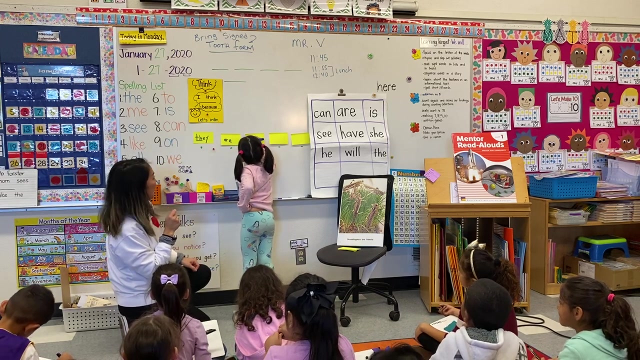 letters make a bruh. Let's want to do brown first, or black. Which word? Brown, Brown, Okay, Brown Bruh, bruh, bruh. What two letters make a bruh, bruh, bruh. What do you boys and girls hear in the beginning? Bruh, bruh, bruh, bruh. Oh, what letter are you going to grab? B, Grab the bicycle, Okay, ready, Throw it in there, Okay, go. You did it. A, B. And then we heard a bruh, bruh, bruh. 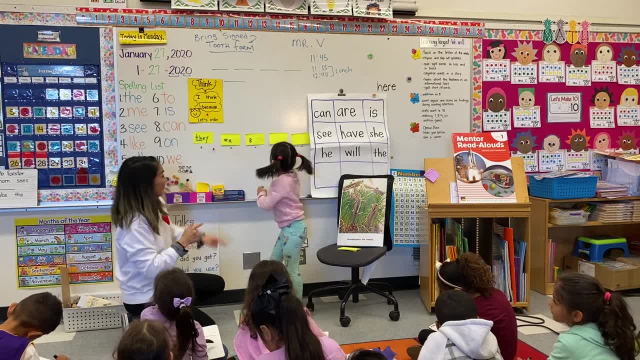 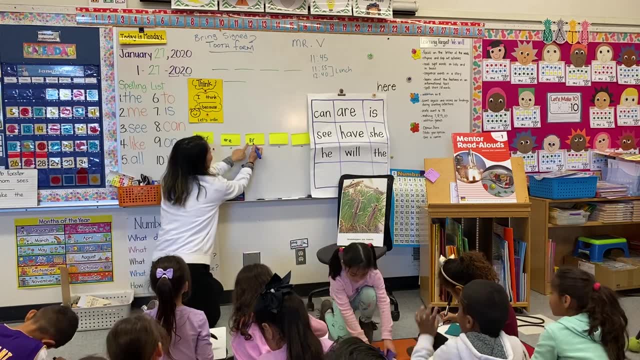 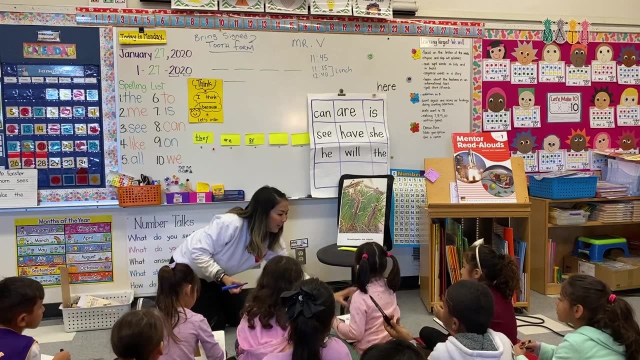 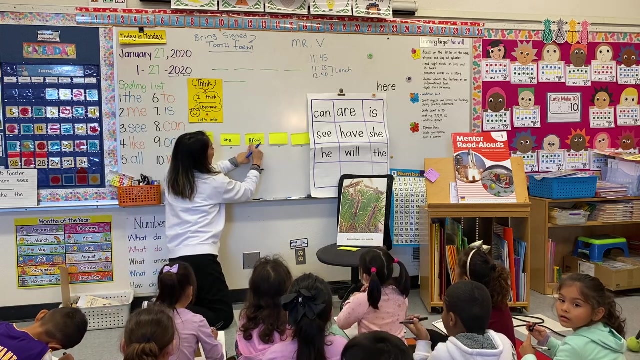 R, R, R R. If you don't know the R, wrap the rabbit and put it next to the B. Thank you, Do you guys see this Brown Brown? Is it not working There? Okay, ready, They are brown. Miss Corky's going to take care of it. They are brown. 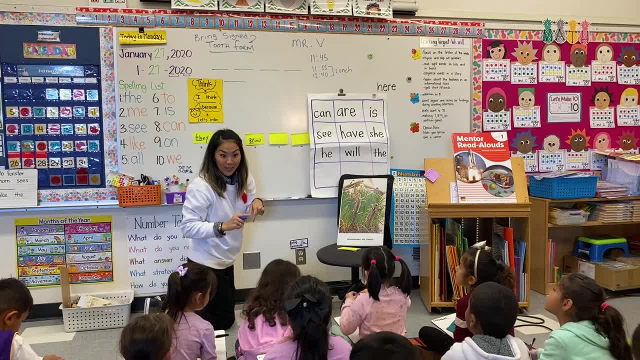 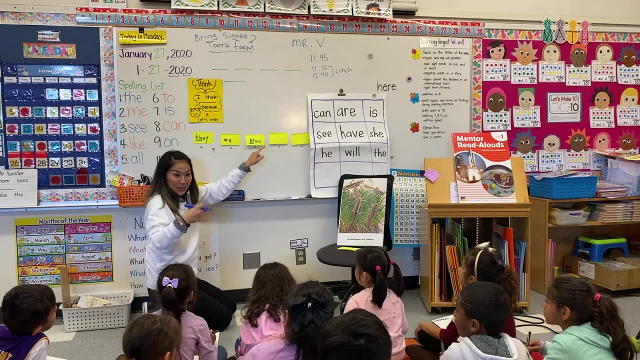 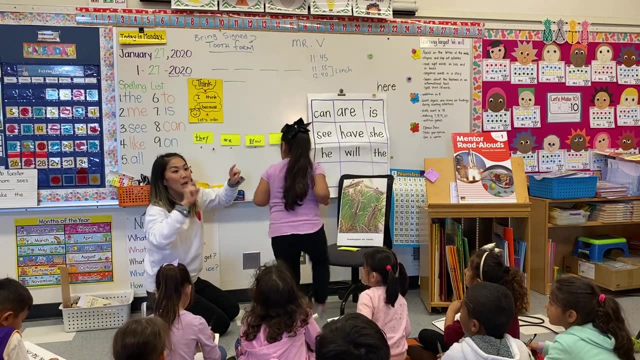 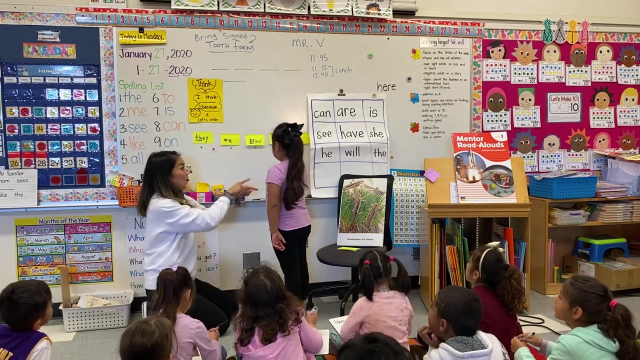 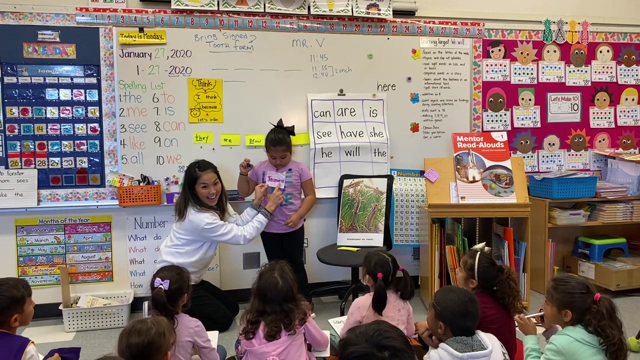 Brown. Jasmine, you have one of the letters, One of the letters in your name. Come on down, Come here, Jasmine, Come, come, come, Come, Jasmine. Jasmine has the letter that I want. I heard a sound here- Watch, Listen, Bruh, Ow, Mmm. What's the last sound? N, N And Jasmine. can you turn around, Jasmine? Look it, Turn around and show it to your friend. Do you see She has a N? Okay, Jasmine. 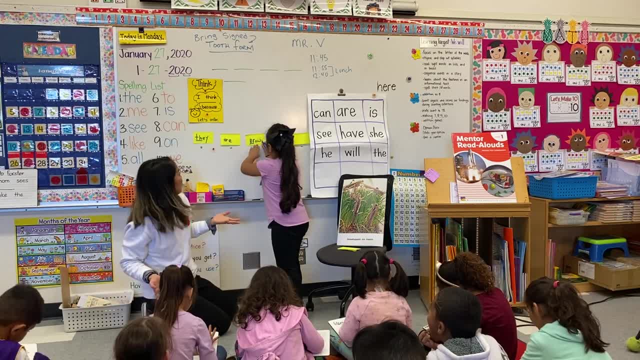 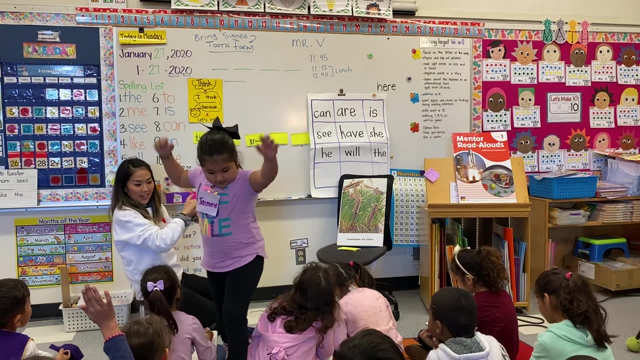 Okay, Jasmine, All right, Do you guys write? And Awesome, A lot of our letters are in our friends' names. All right, Can you put marker up, Marker up, or your little pointer finger up, Ready? Let's go back to re-read it Go. 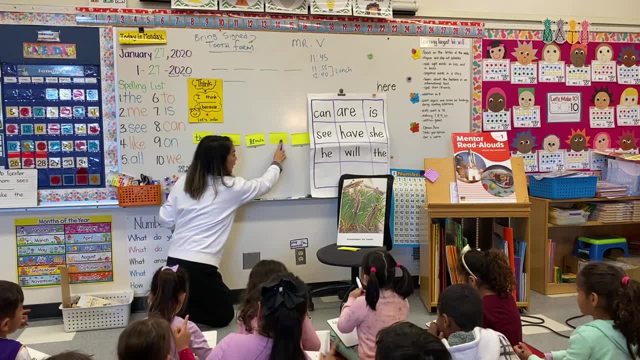 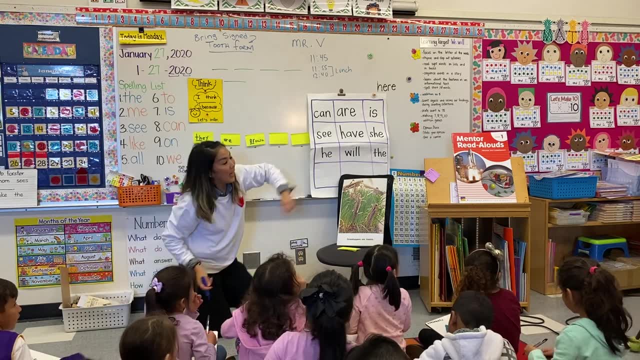 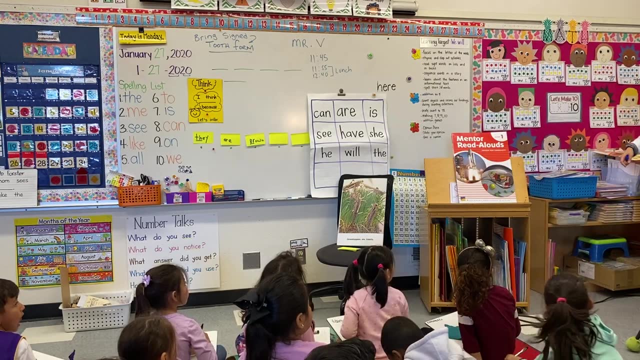 They are brown, And And. Should you know how to spell? and Let me see It's on your pink, Your pink words, right here And the end. How about my friend Isabella? Where's Isabella? Isabella, come find Anne for me. 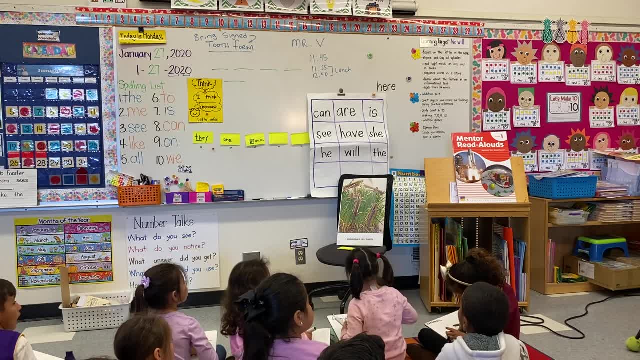 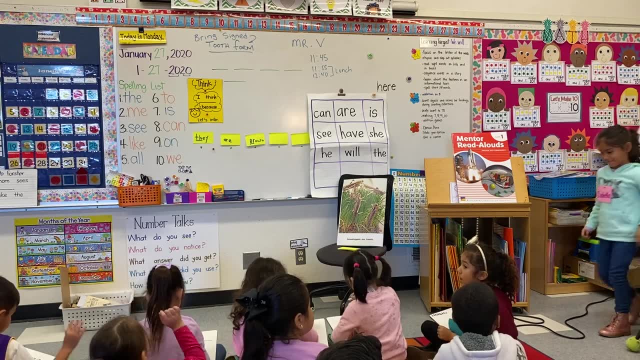 Which one is it? Oh, you got it. Which one? This one or this one? Grab it, Got it, There. Got it, You got it. I got it. Okay, throw it Do it Ready. Okay, Isabella ready. 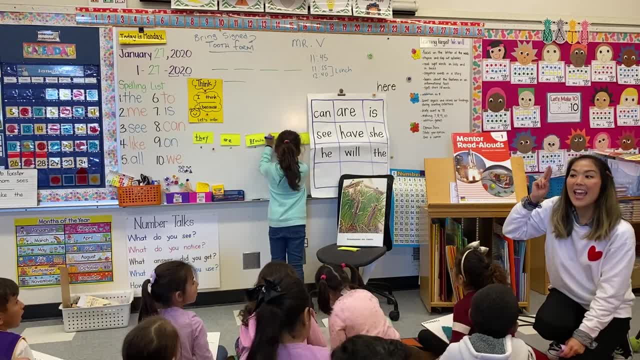 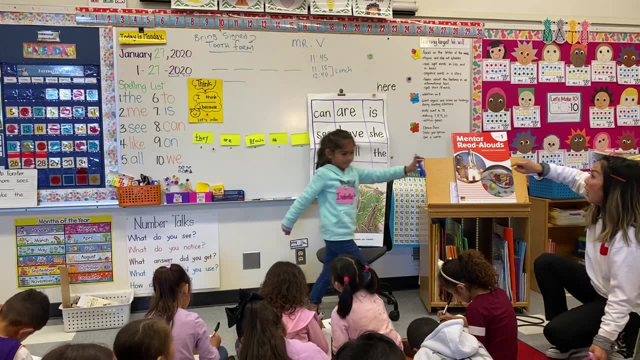 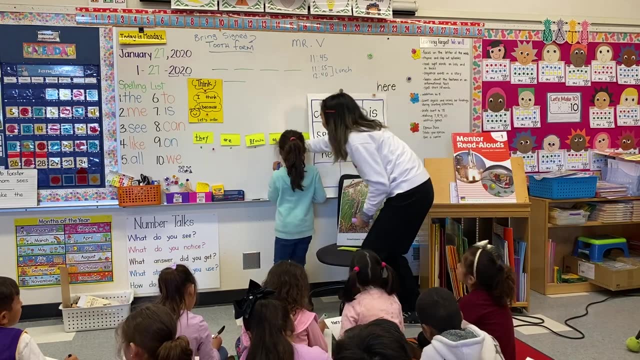 End. How do you spell end, boys and girls, A-N-D. Nice, And if you forget, you can always look there. Oh, Isabella, look, Let's match it. See that A, Let's go? A, B, A-N, Right. 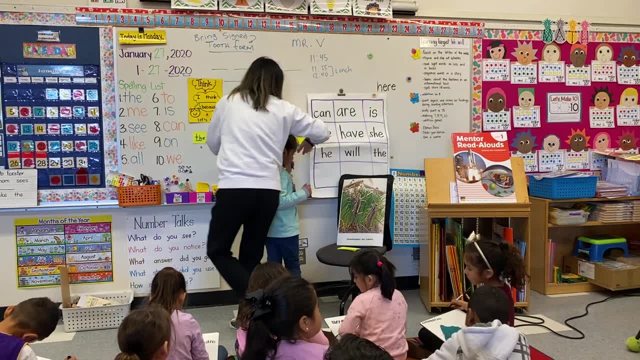 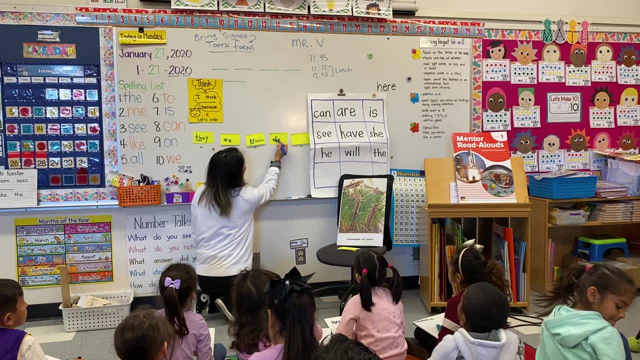 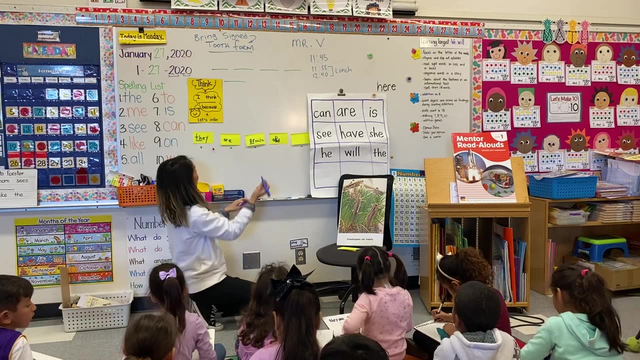 there. Thank you, I'm going to fix your end right here. okay, I'm just going to make it go this way. Okay, Isabella. Okay, Did you guys make it like Isabella's hair? A-N-D. Yes, Yes, Okay. 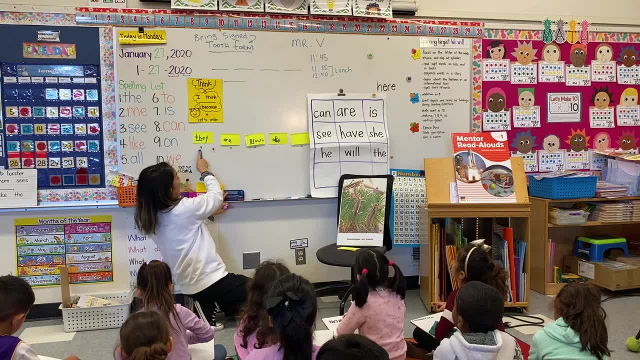 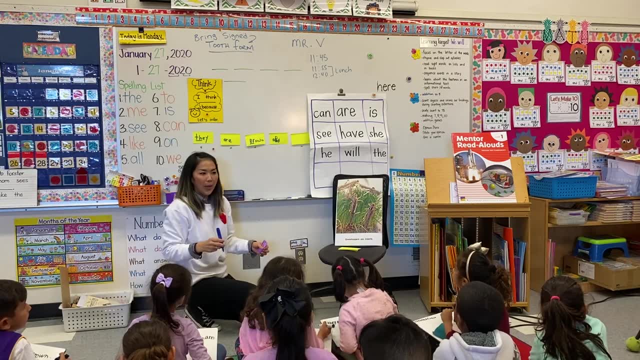 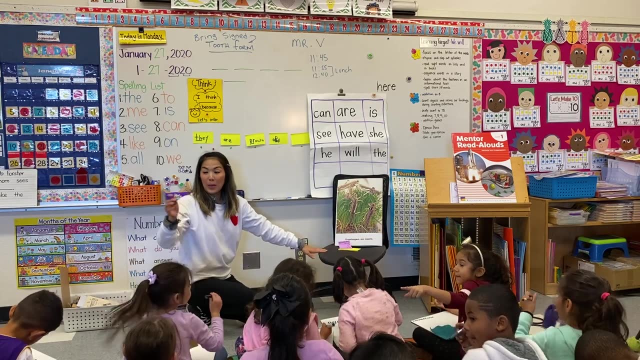 Let's go back, Read it. Hurry, before we get to the last word. Here we go. They are brown and black, Black. Hey, wait, Let two letters make a blah blah Logan. I'm going to call my friend Logan again. Where's Logan Right there? Logan, Ready Blah. Boys and girls. 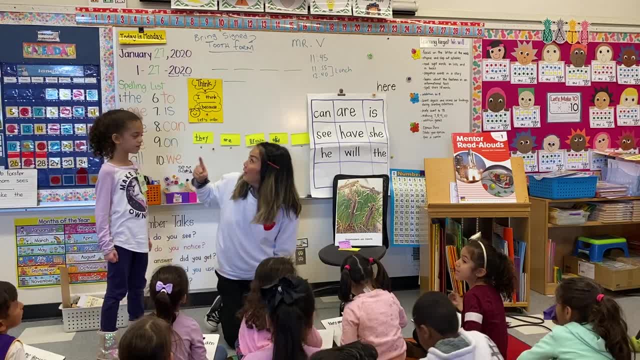 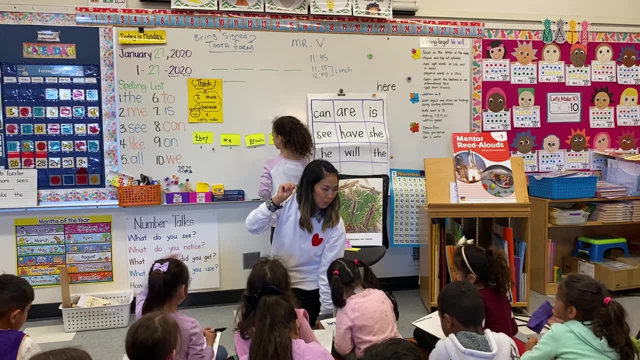 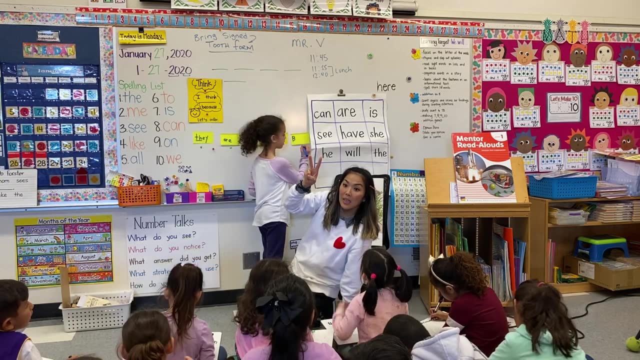 what do you hear in the beginning? Blah, Blah, Blah, blah, B, B, B. Grab the B everyone. Okay, put it right there. Logan, ready, You're going to put two letters together: Blah, ooh, Blah and ooh, Nice Ready. Blah, ooh, Ooh. 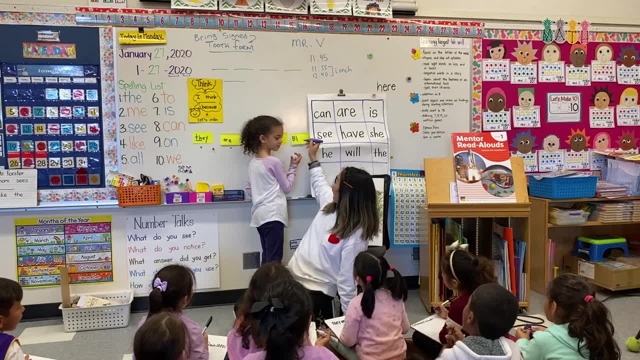 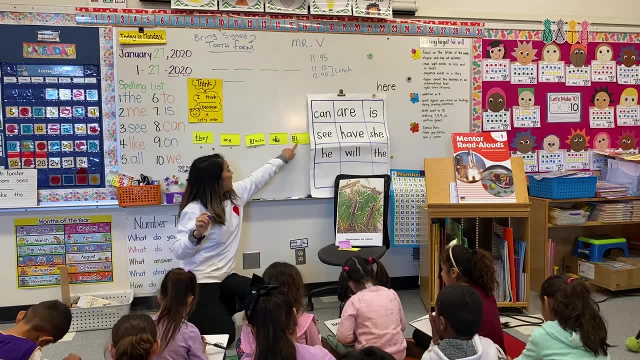 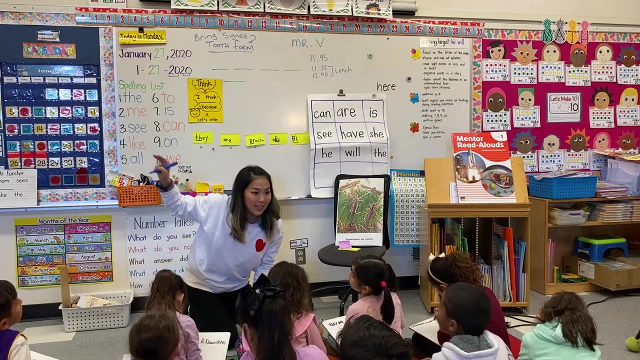 What sound do you hear next? Oh, Did you guys match Logan's? Yeah, Ooh, nice, Ready, Ready, Here I go. I'm going to say the next sound: Blah. Everyone grab the A. Alani has A's in her name. Zaden has an A. Look down in the kitchen. 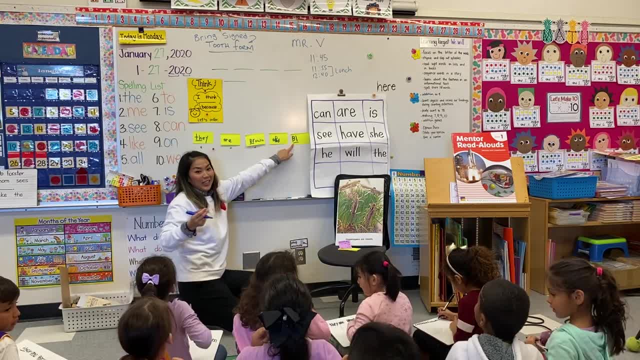 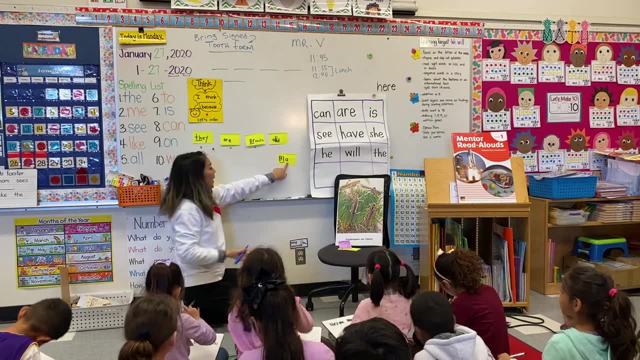 I have an A, You have two A's, I have two A's. Does yours match Ms Courtney's? Yes, Okay, I'm going to take care of the rest- Black- And I'm going to put a period up there. 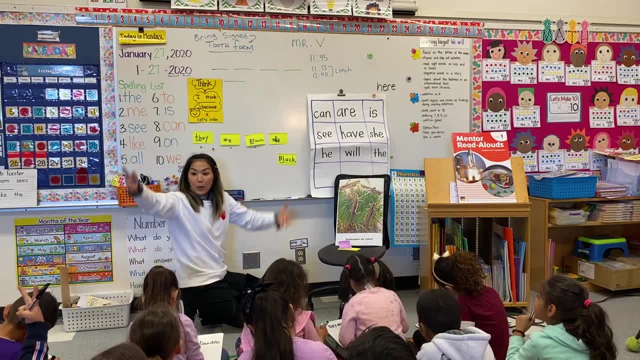 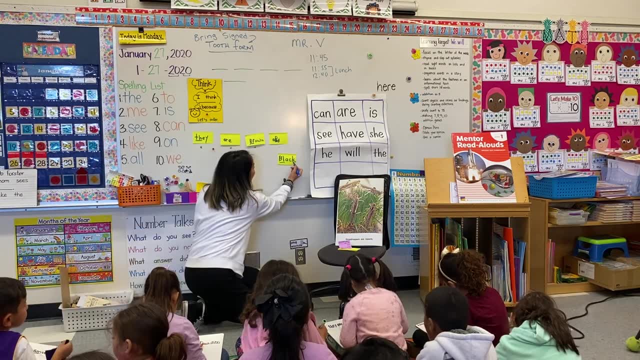 A, that's my name. I have a C of a K. Kaepernick, I should have called on you. I have a C. You have a C. Okay, I have a C. Oh, nice, Okay, Kaepernick, next time. okay, You remind me. I have an A. I have an A in my name. 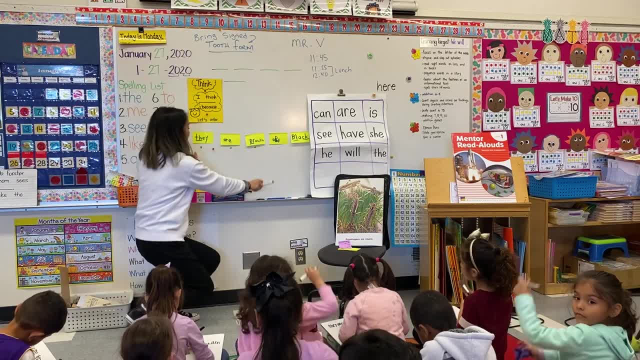 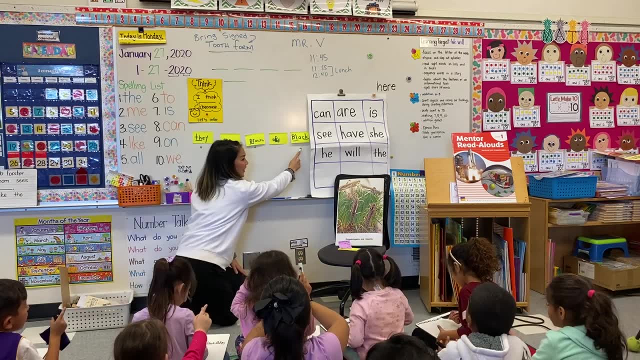 I know, Caleb, You ready, All right, Ready. Markers up, Ready, Or pointer fingers up. Let's go back and read our sentences. Go, They are brown and black. Guess what. You guys are the authors, Just like me. 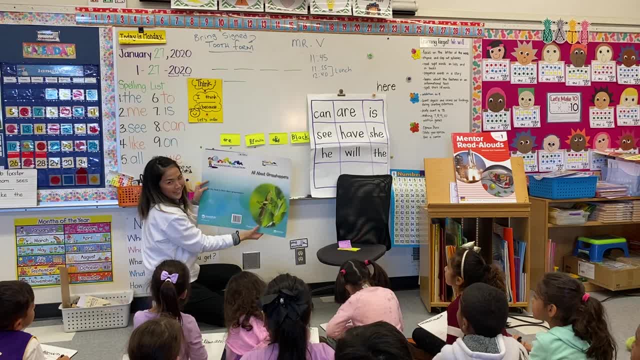 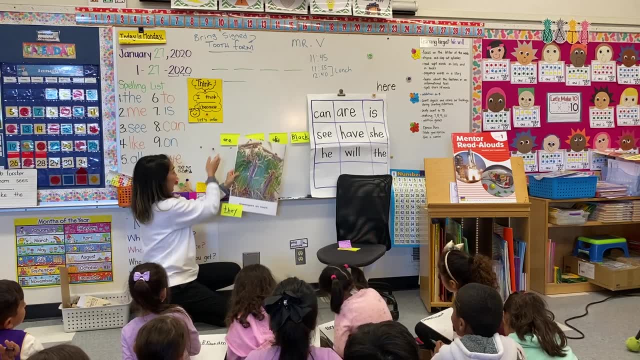 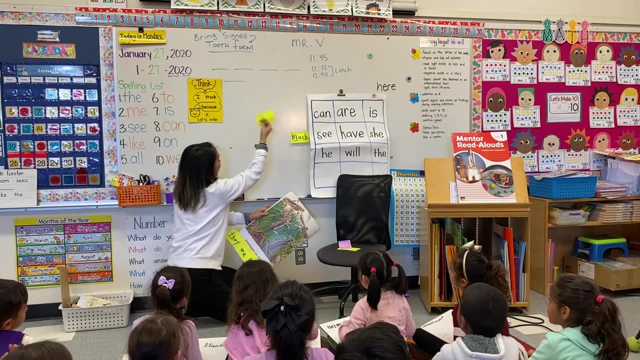 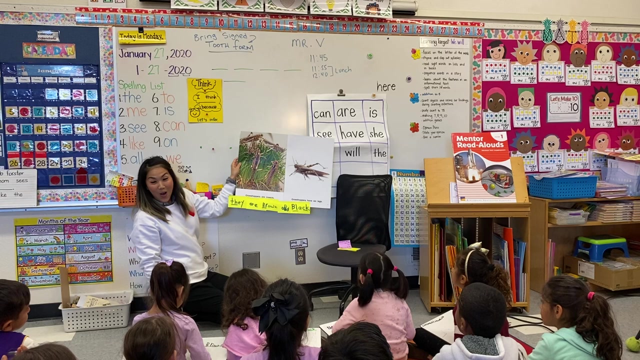 Let me see What was her name: Rhonda McDonald. I get this Watch, watch, watch. Grasshoppers are insects. They, can you read it with me- Are brown and black. Whoa, Do you see how we made our sentence longer?